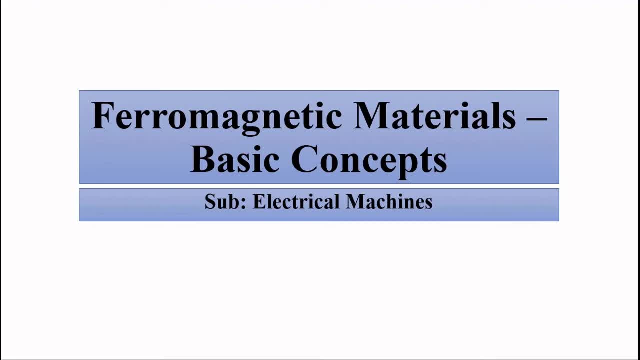 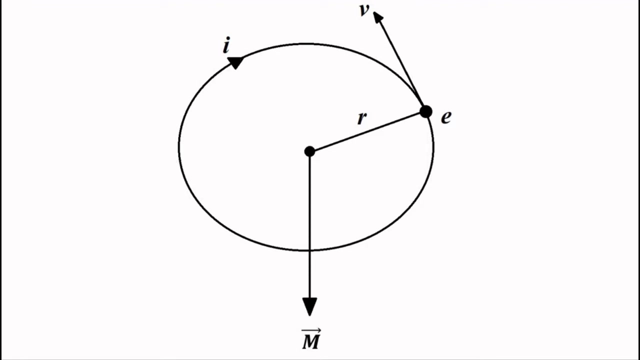 properties of that substance, that object, Either they get magnetized or not. That is, they magnetize in the same direction or in the opposite direction, That is, they acquire attractive characteristics or repelling type characteristics. And it is all due to the movement of electrons in the orbits, resulting in orbital magnetic. 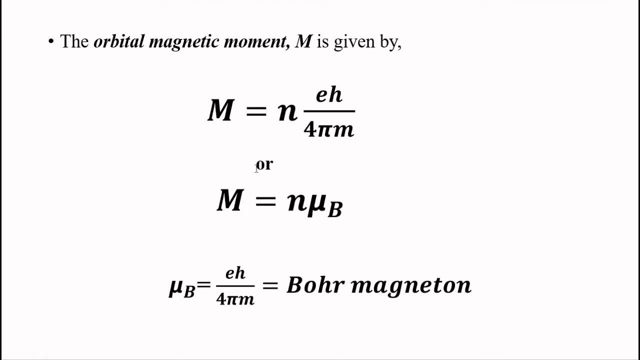 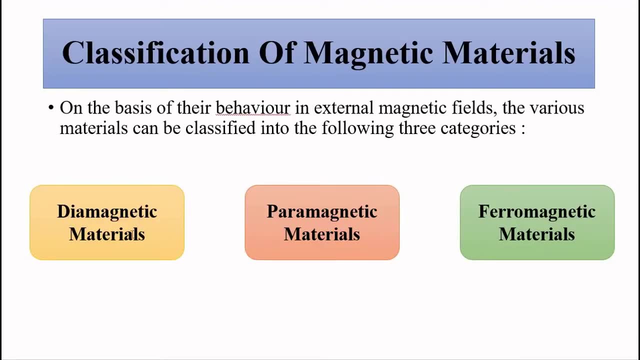 dipole. Okay, And it is because of this the materials. they can be classified into three categories: diamagnetic, paramagnetic and ferromagnetic. Now, there is a lot of similarity between paramagnetic and ferromagnetic. We can say that ferromagnetic is just the. we can say 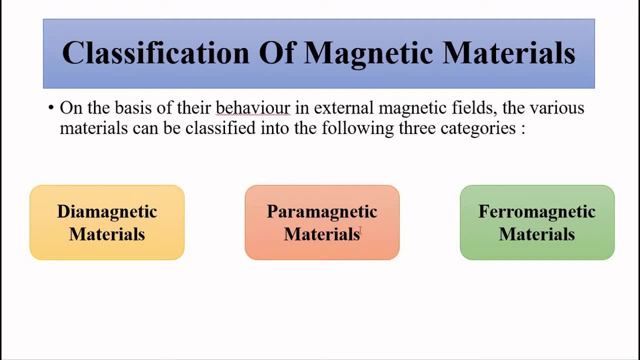 modified version of paramagnetic materials. So ferromagnetic is just paramagnetic in excess. All the properties of paramagnetic materials: when they are enlarged, when the value is increased, the magnitude is increased, it becomes ferromagnetic, So ferromagnetic. 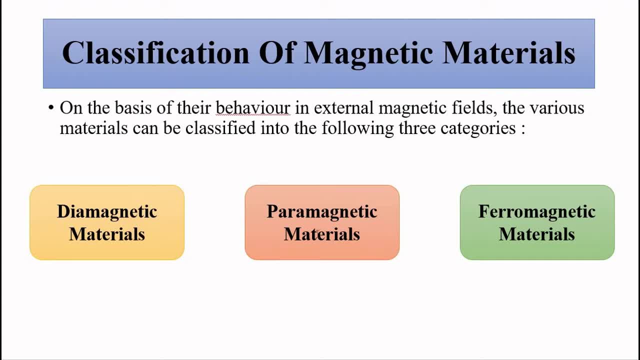 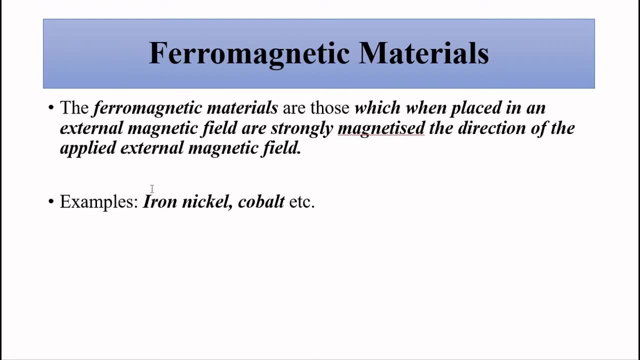 is basically paramagnetic properties in excess or enhanced properties, So ferromagnetic materials. Okay, So ferromagnetic materials are only those residence in external magnetic field. They were those which, when placed in external magnetic field, are strongly magnetized in the direction. 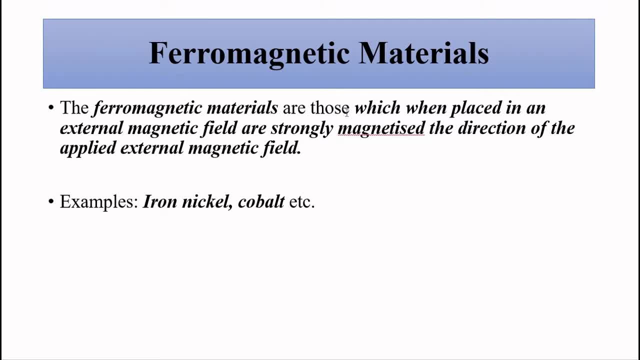 of the applied external field. So now, if you try to remember the definition of paramagnetic materials, it was that these are. they were those objects which, when placed in external magnetic field, are weakly magnetized in the direction of the applied external field. So 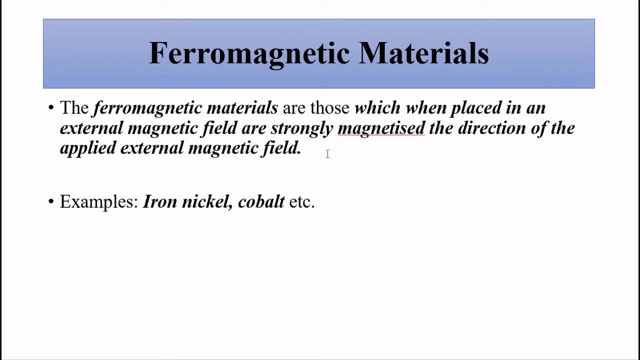 and strongly: Weakly in case of paramagnetic, strongly in case of ferromagnetic. Everything else is the same. That's why I said ferromagnetic is just the magnified version of paramagnetic materials. Example: iron, nickel, cobalt. So these are to name a few examples of 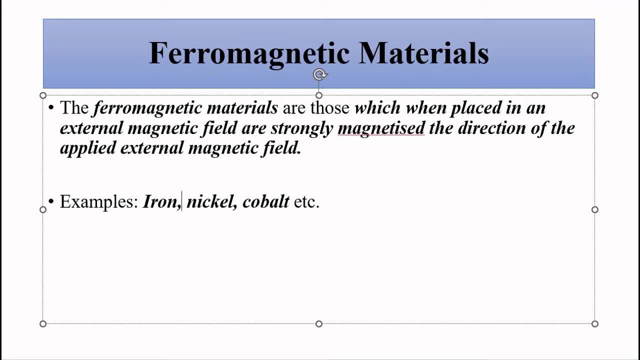 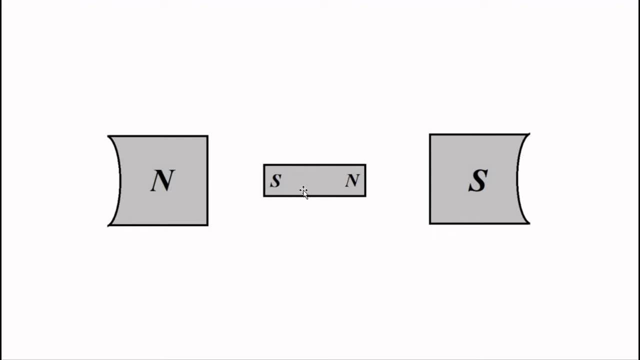 ferromagnetic materials. So the ferromagnetic materials, they behave in the same way, That is, when they are placed in an external field, they acquire attractive type characteristics, which means that the end facing the north pole of the external field acquires south pole. 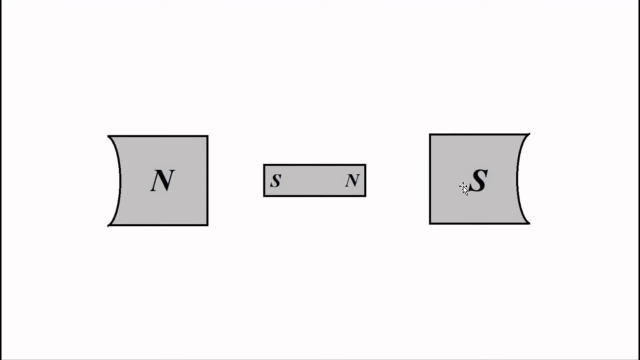 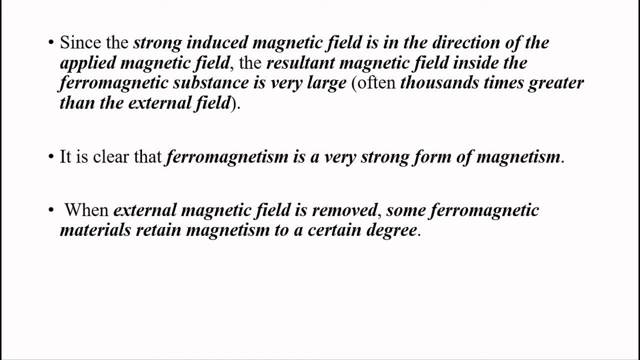 and the end facing the south pole of the external field acquires north pole. That's why it acquires attractive type magnetic characteristics. So the magnetic behavior which is induced in the ferromagnetic material is very, very, very strong. So the resultant field inside 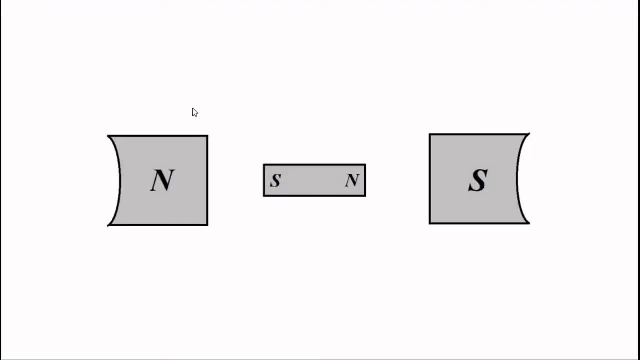 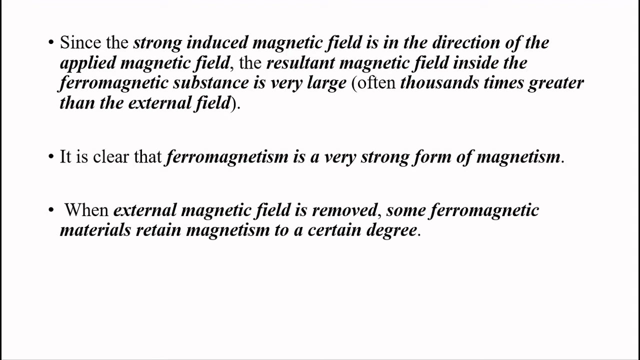 the ferromagnetic material is greater than the external field. In case of paramagnetic it was less. In case of ferromagnetic it is more. Again, magnified version of paramagnetic And opposite to paramagnetic material, it is a very strong form of magnetism and it 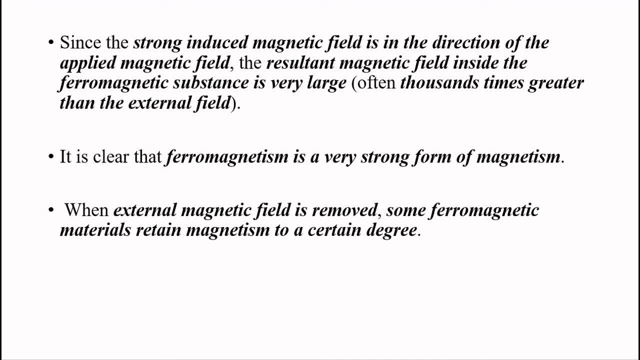 retains its characteristics even when the external field is removed, But in case of paramagnetic, it loses its magnetic behavior. the second: the external field is removed. same the case for diamagnetic, but in the opposite direction. Diamagnetic materials also lose their magnetic repelling characteristics when the external field is removed, but ferromagnetic. 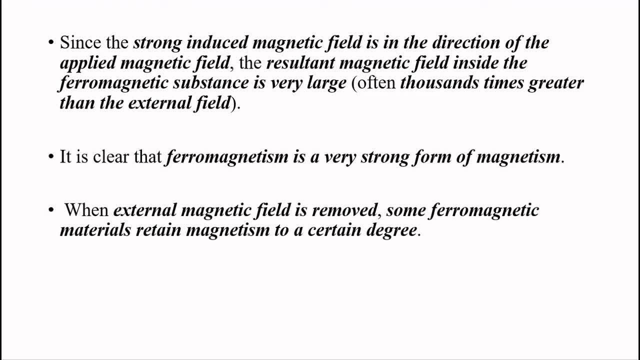 materials. they acquire their attractive magnetic characteristics and they retain it, even when the external field is removed. they retain it to a certain degree. so what is the cause of behavior, this kind of behavior in ferromagnetic materials? so we all know that the magnetic behavior of all materials, be it diamagnetic, paramagnetic or ferromagnetic, it is because of the magnetic 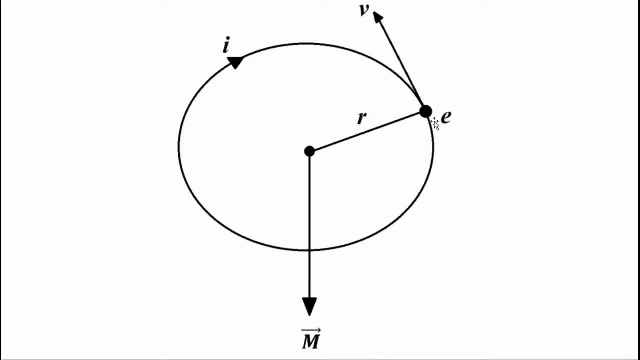 dipole movements because of the revolving electrons, which constitutes a current loop in each orbit and that produces the magnetic moment. the orbital magnetic moment is given by this. now, in case of ferromagnetic materials, a number of magnetic dipole movements. they form groups, okay, they constitute together, they form clusters, they form groups, and each such group is 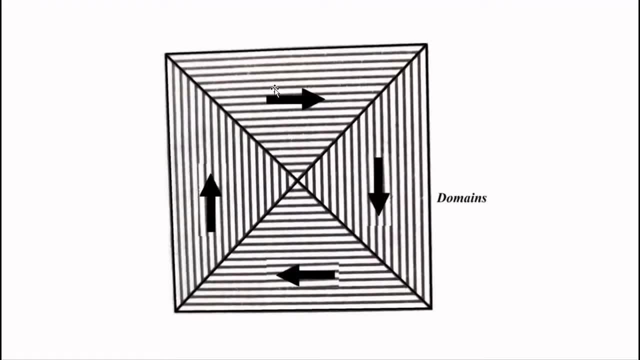 called as a domain like this. so all of these magnetic dipole movements they combine together to form a net magnetic dipole movement, a cluster magnetic dipole movement or group magnetic dipole movement, which is called as domain. but in the absence of external magnetic field, these domains or groups of magnetic dipole movements, they are randomly. 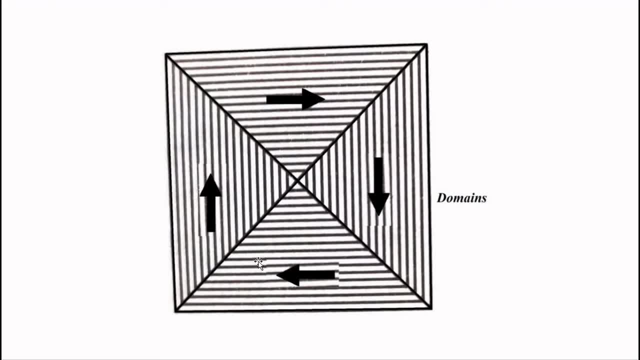 aligned. okay, in random directions. here i've just, you know, like this i have expressed, but it can be in any direction. the arrowhead can be in any direction. there are many different directions. they are not in one direction and these big arrowheads are nothing but to represent group or 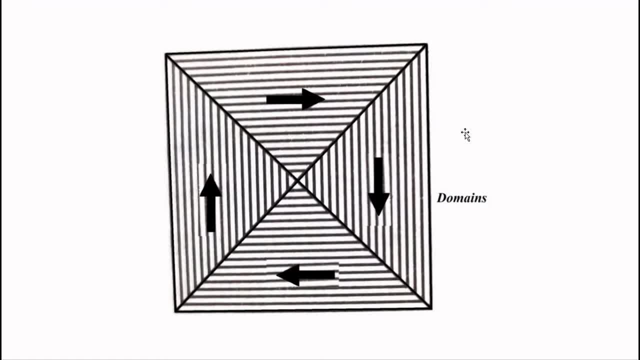 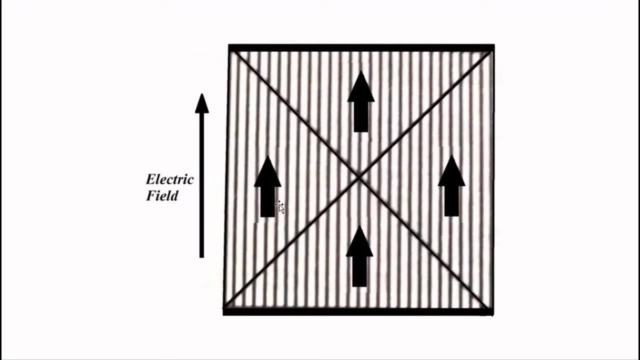 cluster of many magnetic dipole movements. this is, in the absence of external field, randomly aligned, randomly directed. but when they are placed in an external magnetic field, these domains or clusters of magnetic dipole movements or group of magnetic dipole movements, they align themselves in the direction of the external magnetic dipole movements and they are not in one direction. 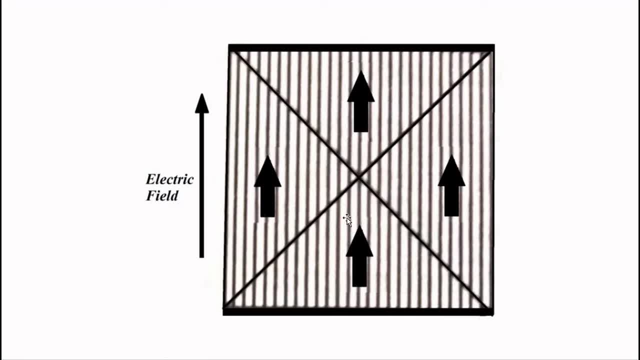 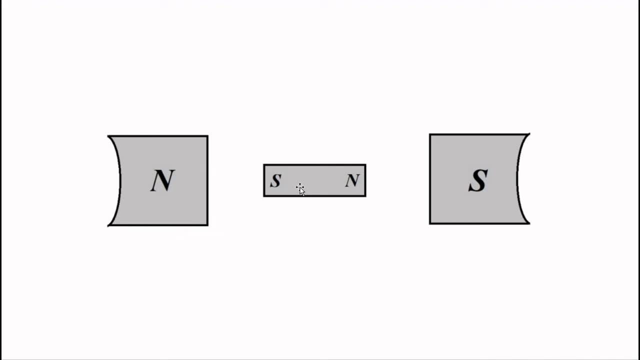 they are directed in that direction and it is because of this property that ferromagnetic materials, they acquire attractive type magnetic characteristics, but in a strong way, okay, in a strong way. in case of paramagnetic, the number of such magnetic dipole movements were was very less. 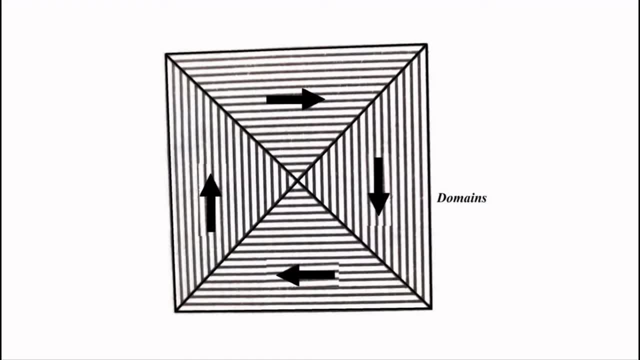 it was not as huge as the ferromagnetic case. that's why, because of this, the less number of magnetic dipole movements- paramagnetic type attractive characteristics is very weak in nature, but ferromagnetic type attractive behavior, attractive magnetic characteristics is strong in nature because of the more number. 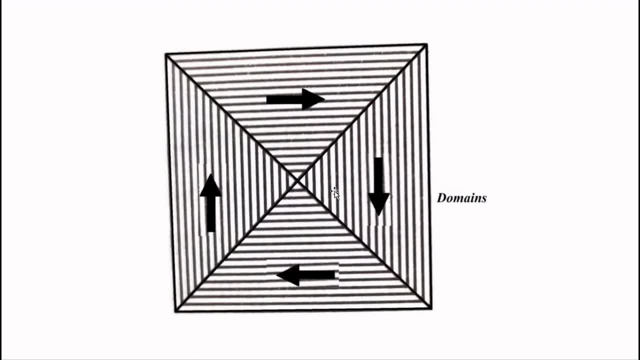 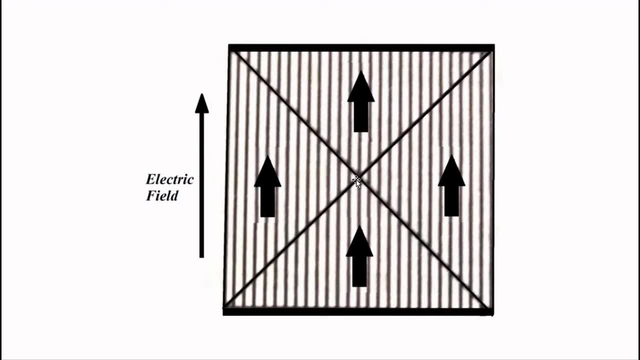 of magnetic dipole movements. okay, so it is because of this, domains getting directed in the direction of the magnetic field, the magnetic dipole movements tend to be faster than they field, and the more number of such cluster or grouping of magnetic dipole moments in one direction, ferromagnetic type behavior, is attractive in nature and is very strong. 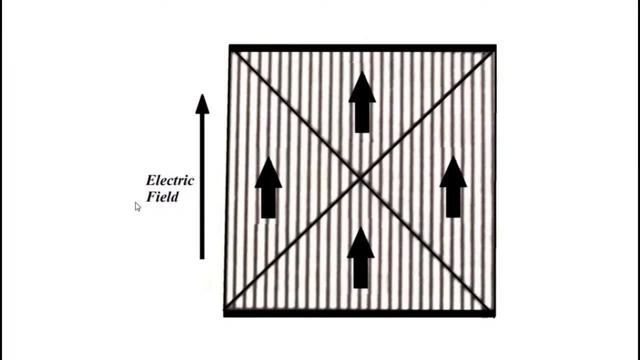 so, friends, here it is not electric field, it is actually magnetic field. by mistake, i have written here electric field, so please, i'm sorry for that. i've made a mistake. so please note that this is not electric field, it is magnetic field. the direction of the magnetic field and the domains. 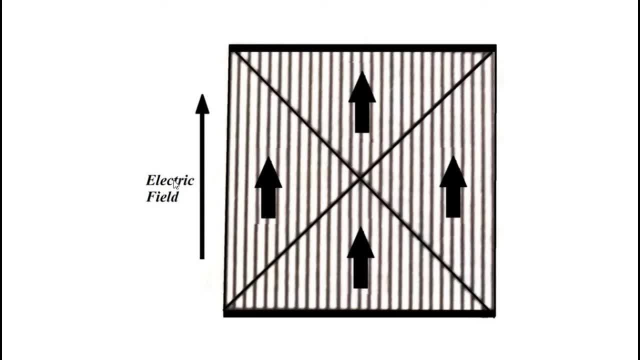 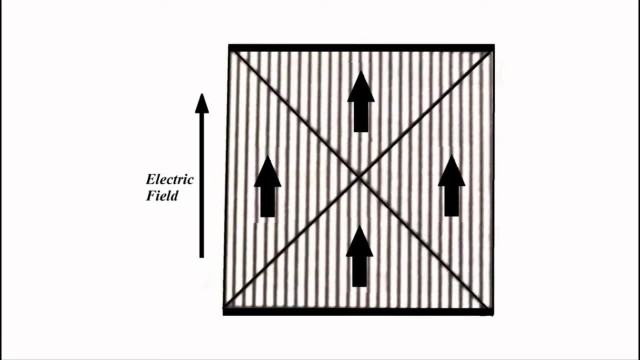 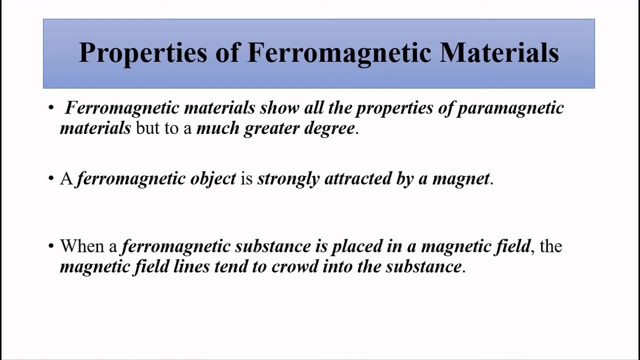 are aligned in that field. okay, so i apologize for the mistake. it is magnetic field, not electric field. so some properties of ferromagnetic materials, very similar to paramagnetic, but just magnified. everything, every aspect is magnified ferromagnetic materials. like i said, they show. 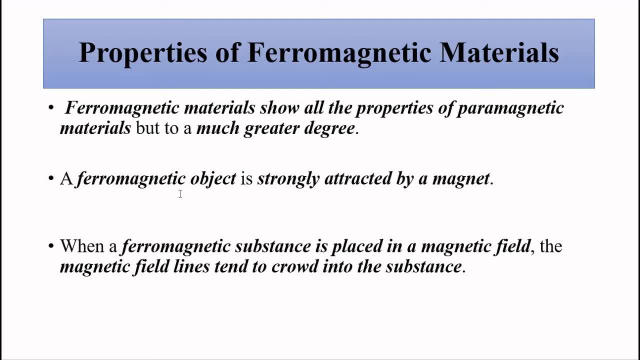 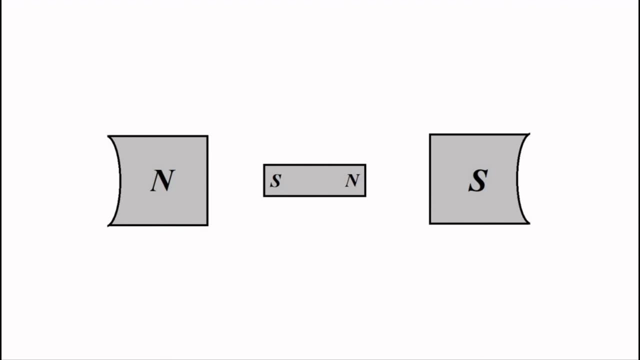 all the properties of paramagnetic materials, but to a much greater degree magnified. everything is magnified. ferromagnetic object is strongly attracted by a magnet because of opposite nature of poles facing each other. but here the attractive, the attraction is very large. okay, because of, again, like i said, the domain behavior. 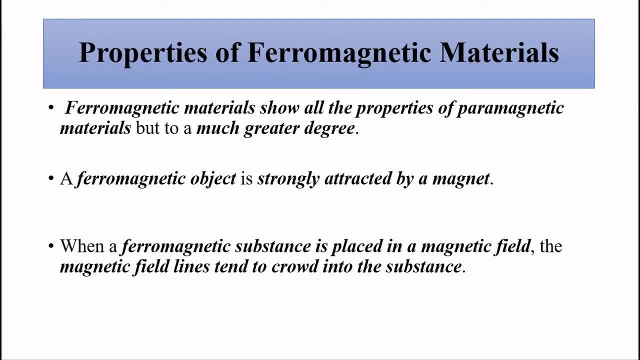 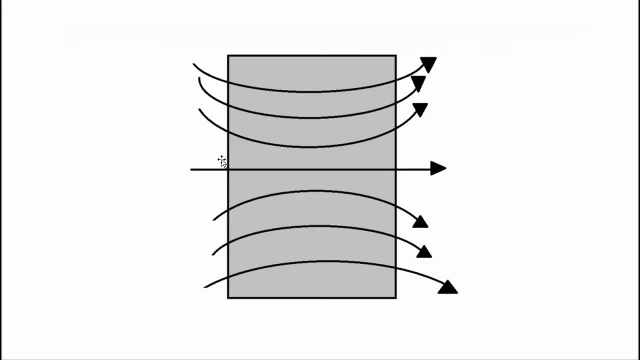 then uh. in case of ferromagnetic materials, when it is placed in an external field, more number of magnetic lines of force pass through the material. but in case of paramagnetic, the number of such magnetic lines of force was less. so again, magnified version of paramagnetic behavior when uh. 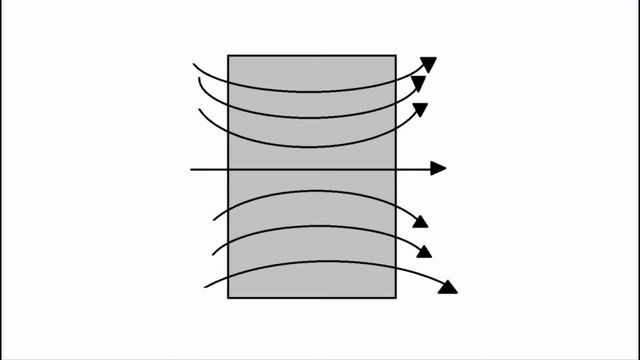 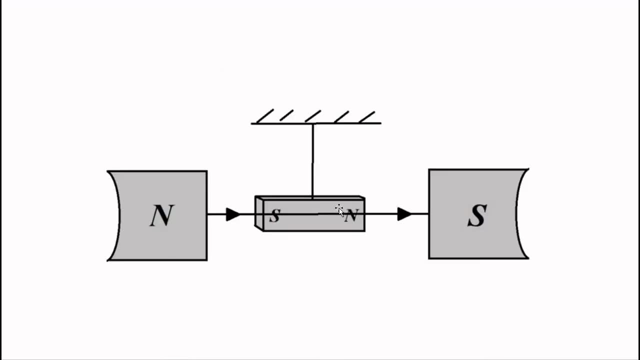 ferromagnetic material is placed in an external field. a rod kind of or a bar of ferromagnetic material is placed in external field. the longest axis: it aligns itself in the direction of the magnetic field, similar to paramagnetic, but it does it quickly. the difference between paramagnetic and ferromagnetic is that in case of paramagnetic, 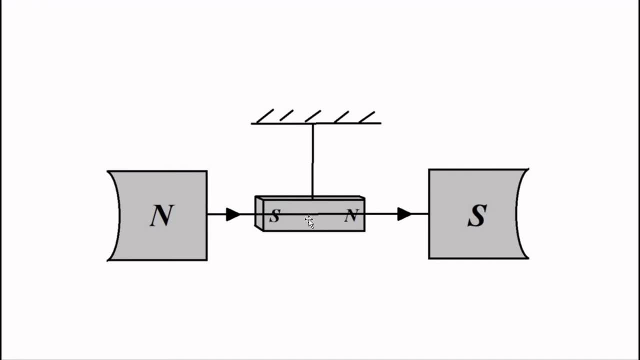 material, this position, this alignment of position in the direction of the magnetic field. it takes slowly because of the weak, attractive nature, weak, attractive magnetic behavior in case of paramagnetic. but in case of ferromagnetic this alignment happens very quickly. the moment it is placed in the magnetic field it quickly aligns itself in case of paramagnetic. 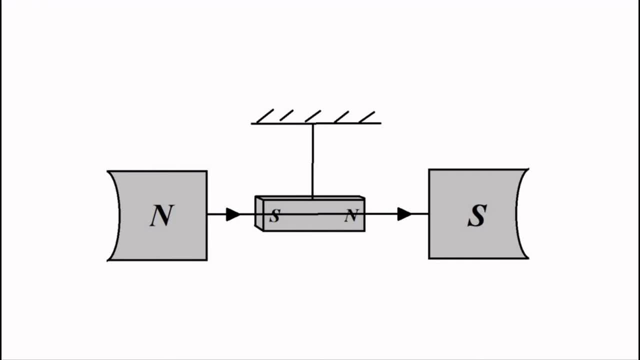 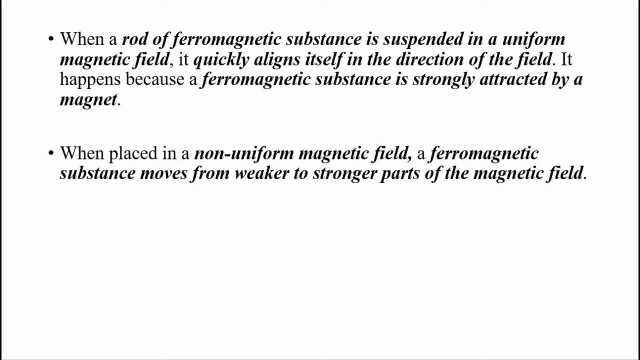 this is very slow. then when it is placed in a non-uniform magnetic field it moves slowly from weaker to stronger parts of the magnetic field- the paramagnetic thing- but in case of ferromagnetic it moves quickly from weaker to stronger parts of the magnetic field because of 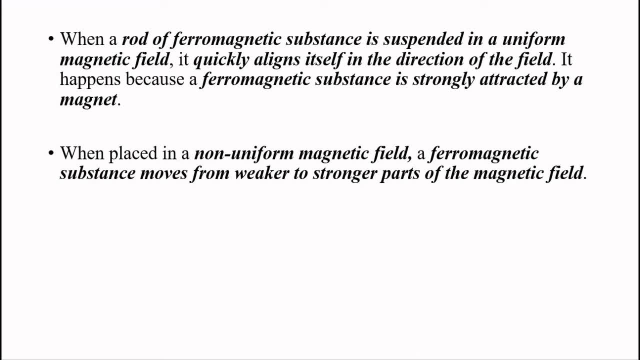 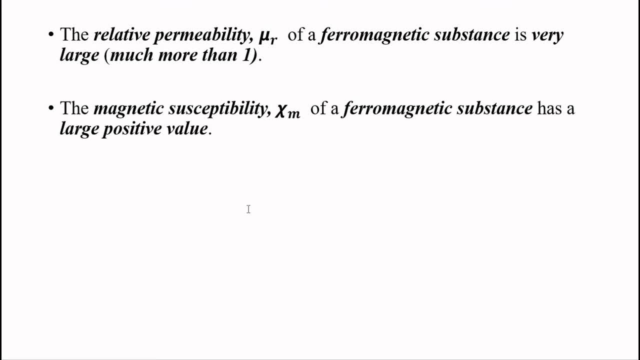 the attractive case then. the permeability of ferromagnetic material is very large, much, much, much greater than one. in case of paramagnetic, it was just greater than one, just not much. also, the susceptibility has a large positive value for ferromagnetic material, but for paramagnetic it was a small positive value. 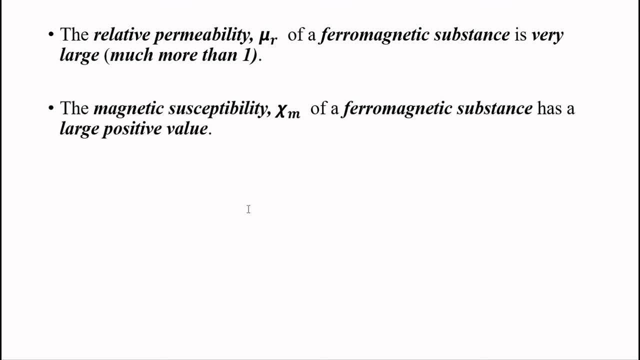 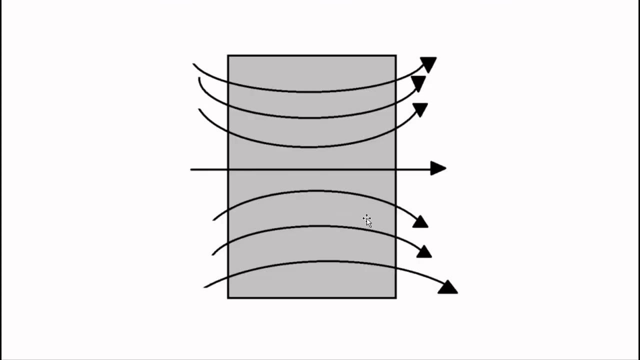 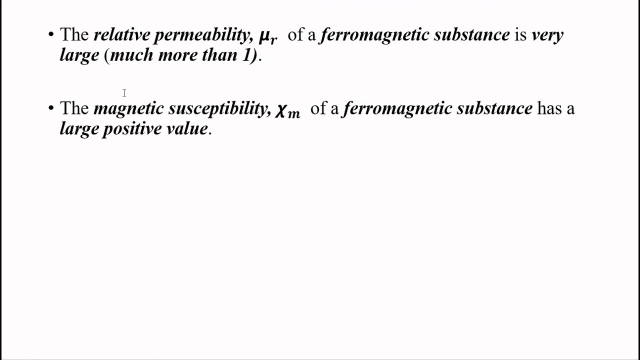 just greater than zero. so, like i said, all the properties of ferromagnetic materials. they're similar to paramagnetic materials, but they are just magnified in every aspect. more number of magnetic lines of force pass through the material, then magnetic susceptibility has a high positive value. magnetic permeability is much greater than one. then it quickly aligns itself.